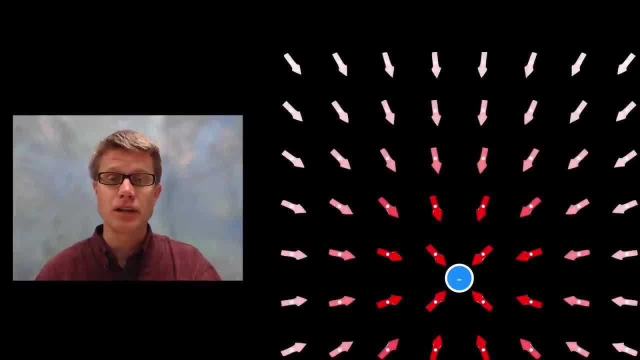 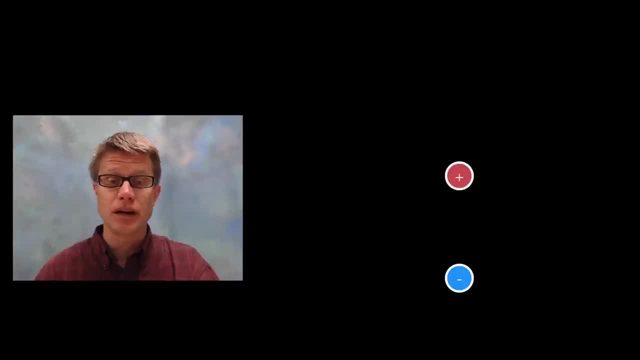 were to take a negative charge like this. we are going to have all of those electric field lines pointing in, And so our equipotential lines would look like that. What if we had a positive and a negative charge? What would the electric field look like? Well, we would. 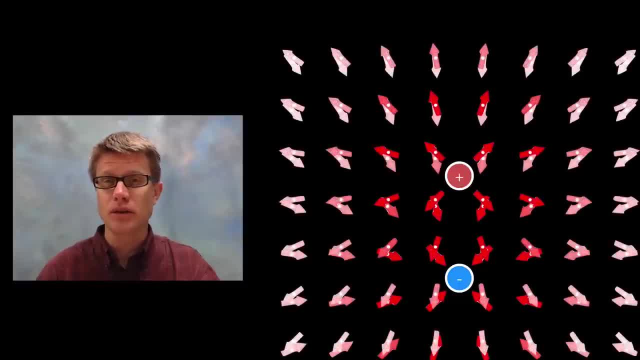 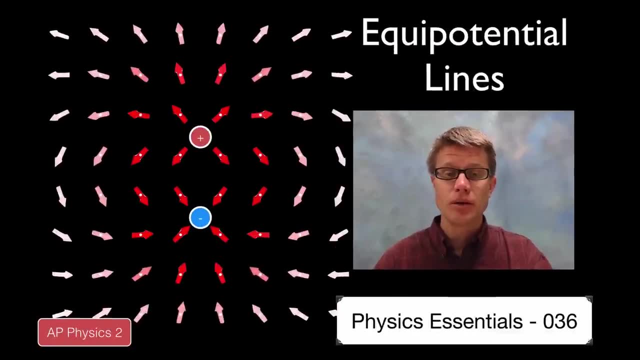 have to combine that of the negative and the positive, So you would have to do a little bit of vector addition. But we would get electric field lines that would look like this: Where are those equipotential lines going to be? Well, they are going to be a little more difficult to draw and they would look something like: 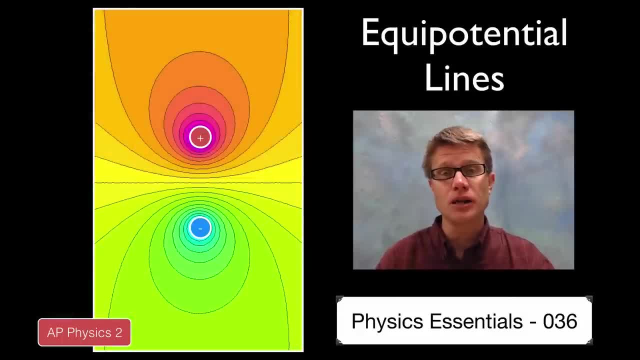 that, And so equipotential lines. in the last video, we talked about contour lines that show lines of equal elevation and therefore equal gravitational potential energy. Well, we are going to use that as an analogy to explain what is really going on. if we are looking, 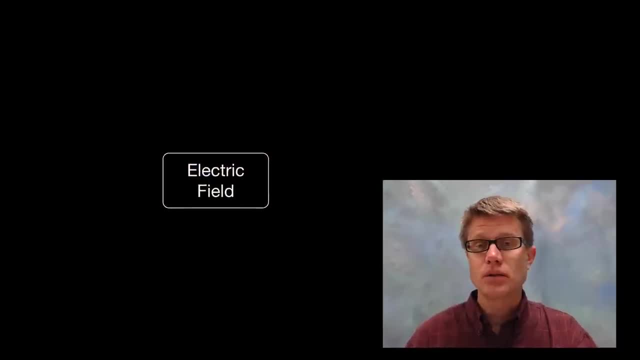 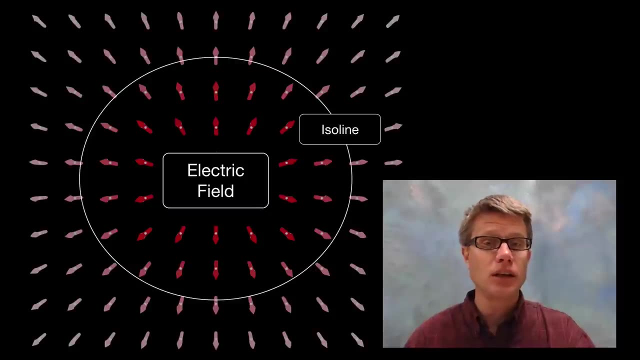 at areas of equal electric potential. And so if you have an electric field and we have these electric field arrows representing the electric field, An isoline is going to be lines of equal electric potential, An equal potential, and that is why we call them equal. 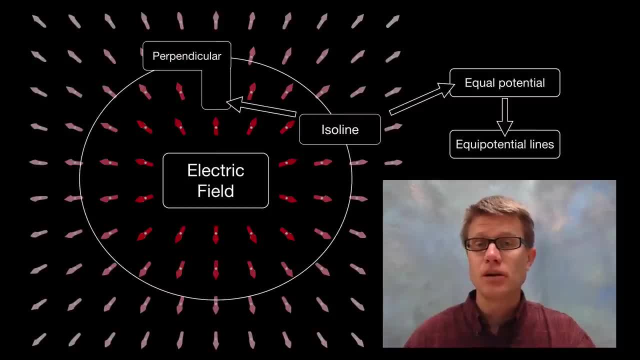 potential lines, And so one thing you should note is that they are always going to be perpendicular to the electric field. And so if I look at, for example, this electric field right here, you can see it is pointed in the downward direction and we can see it is totally perpendicular. 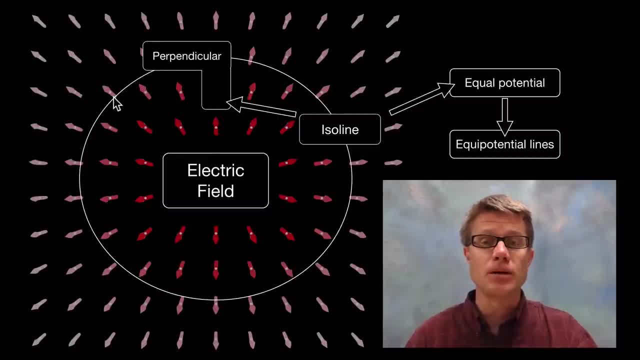 to that and to that and to that, It is always going to be perpendicular to the lines of the electric field. And so if we take a test particle, if we take a positive particle and we're moving it against the electric field, remember we're going to have to do a certain. 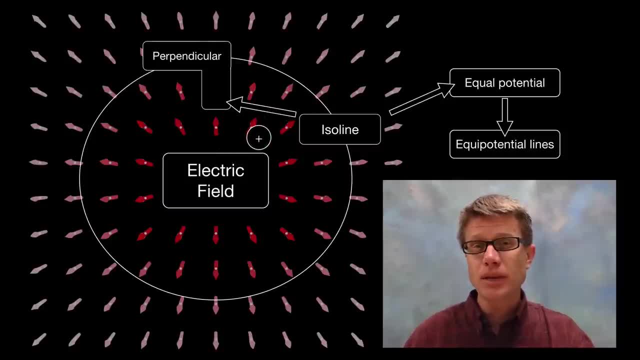 amount of work to move it in that direction. But a take home message you should get is: if we take a test particle like this and we move it along the isoline, since the potential energy is never changing, it requires no work to do that. It's kind of like walking along. 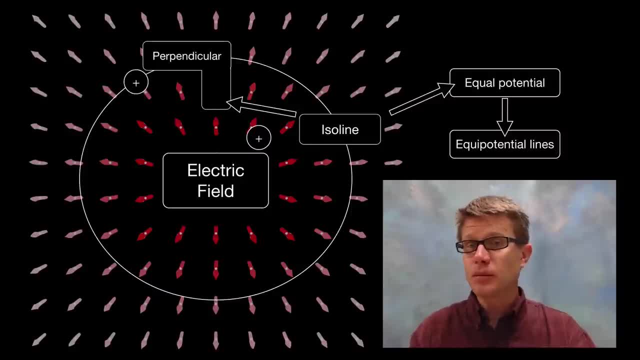 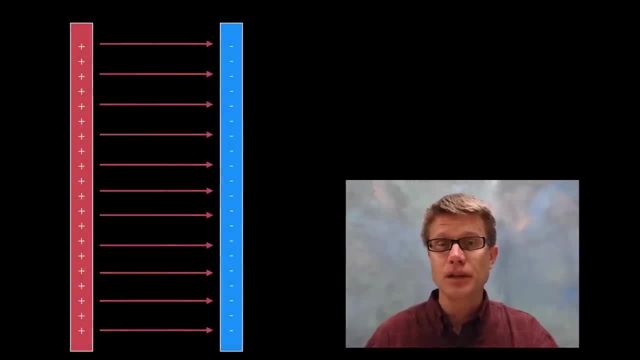 a mountainside, but you're staying at the same elevation. Now you might be spending energy to move in the horizontal, but you're not spending any energy to move in the other direction. And so if we've got two parallel plates like this, we've drawn the electric fields and 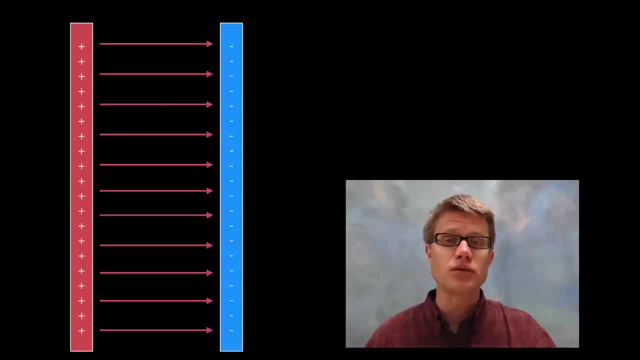 we've talked about that. Do you remember how the potential is going to differ as we move across that gradient? Well, again, it's not, And so we would draw those equal potential lines like this: In other words, it's going to be the same slope, It doesn't matter where. 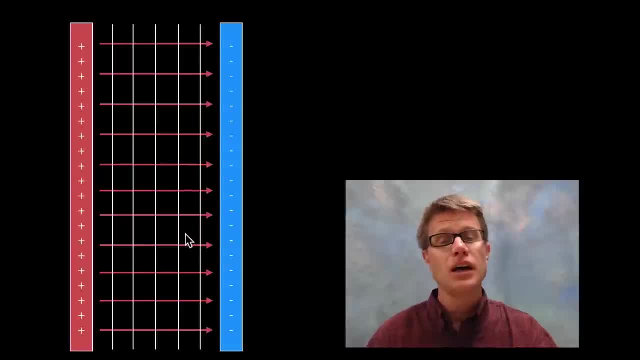 we put it, It's going to be the same potential difference between the two sides, As long as they're close enough together in relation to the length of the overall parallel plates. And so you can think about that, And so you can think about that, And so you can think. 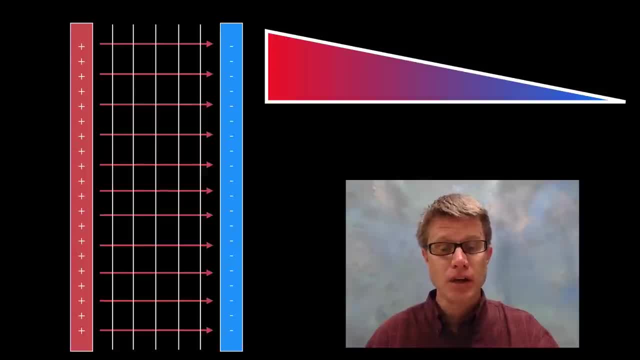 of this almost like an inclined plane, And so since these lines are equally spaced, then the slope is going to be consistent. from the left side to the right side, We're going in the direction of the gradient, And so if we were to take a ball and put it at the top, 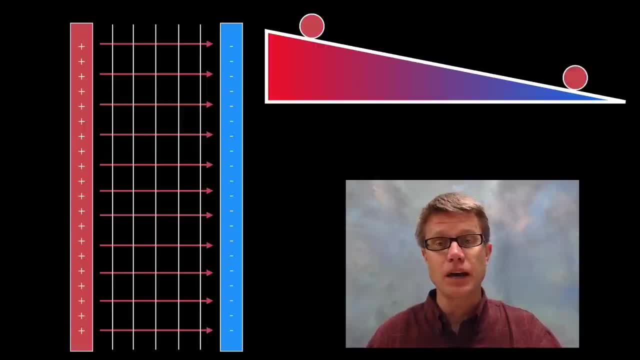 it's going to experience the same potential as a ball, that we put it farther down. And likewise, if we're going to move it up, we're going to have to do work in this direction to move it that direction, But it's going to be a consistent amount of work as we move. 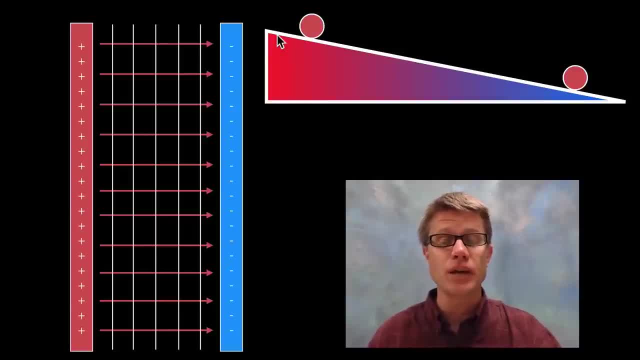 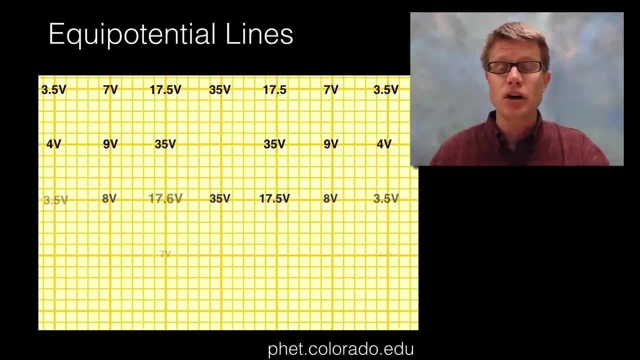 up, And so this is a consistent electric field And therefore we have consistent equipotential lines. So now let's look at an electric field that isn't consistent throughout. So imagine we put a charge right here in the middle, So we're going to put a positive charge here in the middle. If we were to draw equipotential 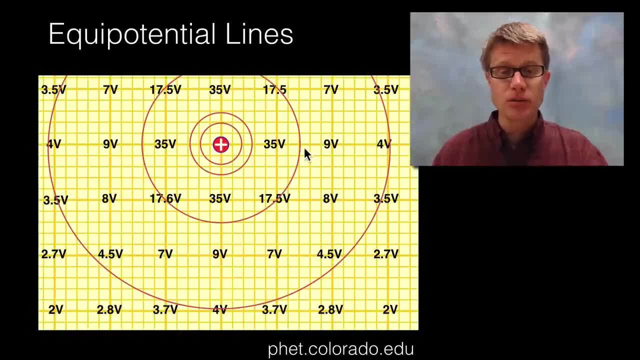 lines, they're going to look like concentric circles. But again, the closer we get to that test charge, we're going to see an increase. This is that inverse square of the radius Coulomb's law. And so if I were to represent this three dimensionally- and this is my best- 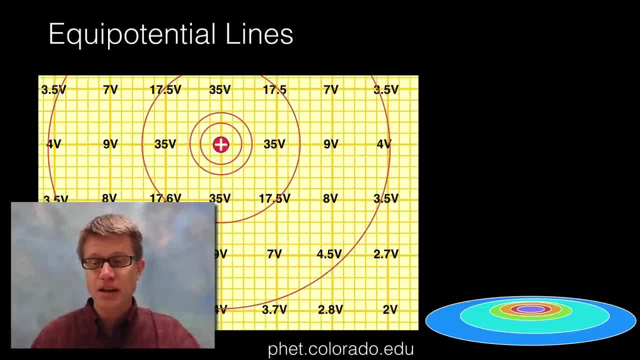 try. I drew a bunch of concentric circles like this. And then I drew a bunch of concentric circles And now I'm going to simply lift those concentric circles to the potential that they're at And I'm going to project it like that. So what we get is a three dimensional. 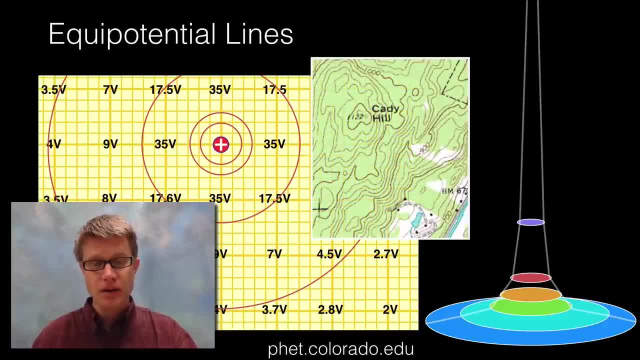 progression, And really what we're showing is a topographic profile. The closer we get to that charge, the higher the potential energy is going to be, And so you can think of putting a test charge here on the side of it is like putting a ball on the side of a hill. It's. 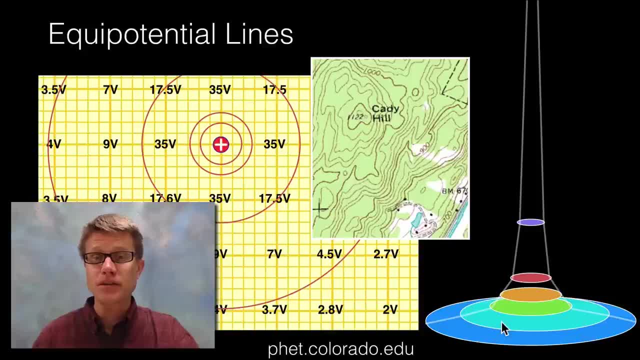 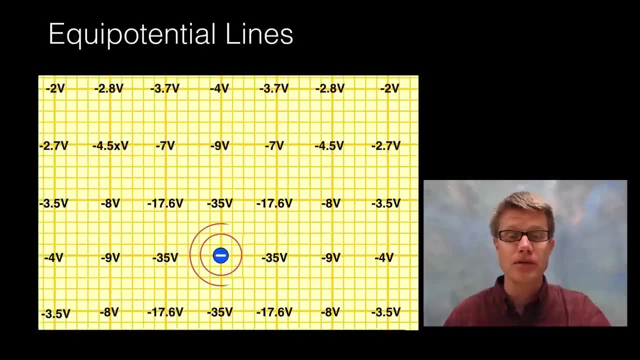 going to move down And so it's going to fall at a faster rate when it's close to that positive charge. Let's say we try a negative charge. We're going to get a similar relationship like this If we were to graph those concentric circles again in three dimensions and we project them. 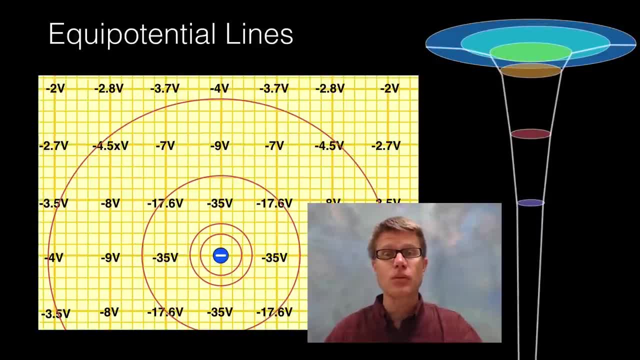 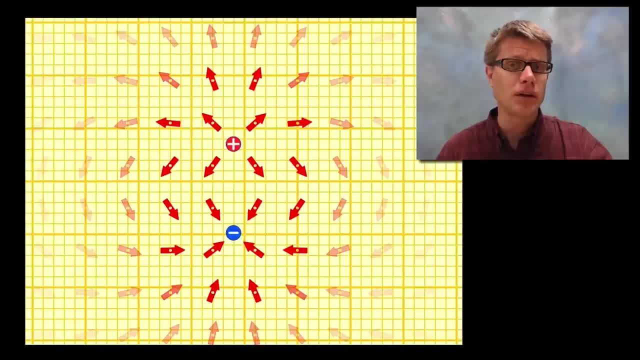 it's going to be like a giant hole, And so if you put a test charge on the side of that, where is it going to go? It's going to spiral in to the inside of that. What if we had something like this, though: If you're given a bunch of electric fields and you have to figure,